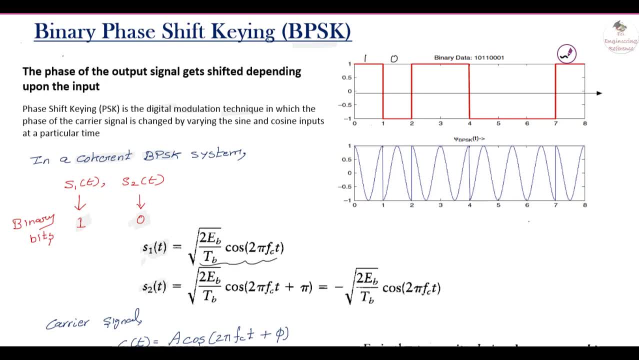 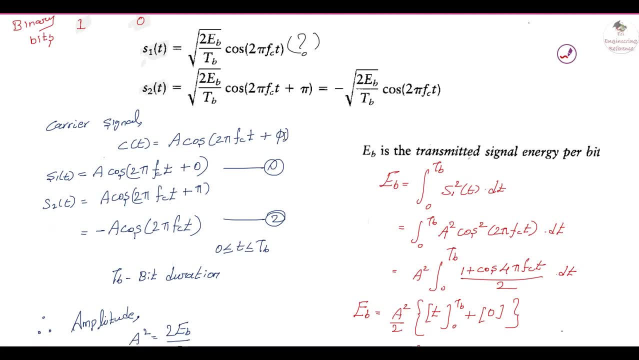 by tb into cosine of 2 pi fct, and s2 of t is the negative value of the signal. So basically, the carrier signal which carries the information bits we consider in every modulation technique is: c of t is equal to a into cosine of 2 pi fct plus 5.. For the information bit 1, that s of 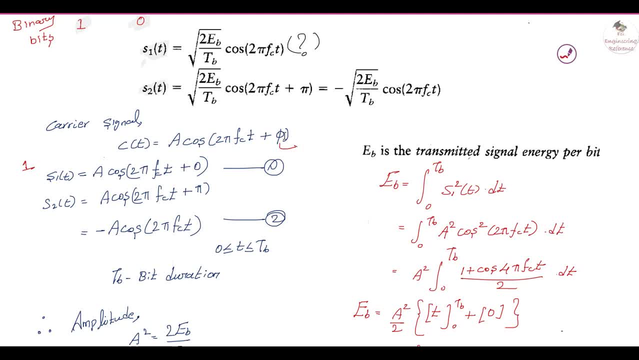 t, the carrier is as it is and the phase angle is taken as 0 and to transmit the information, bit 0 s2 of t, where the carrier signal phase angle is kept: 180 degree 5.. So we know a cosine of 2 pi fct plus 5 is minus a cosine of 2 pi fct. 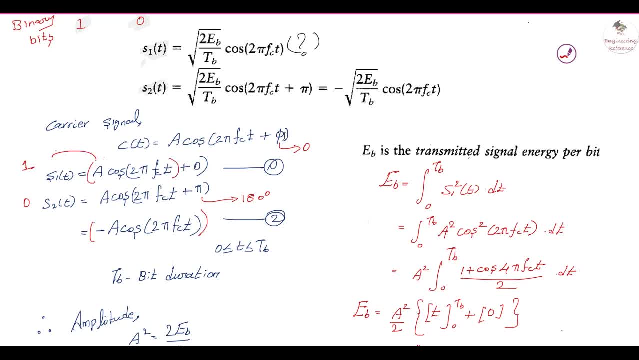 So in this case we have to substitute the negative term. a cosine of 2 pi fct is representation of the symbol 1 and minus a cosine of 2 pi fct is the representation of symbol 0. And under the interval of 0, less than or equal to t. less than or equal to tb, tb is the bit. 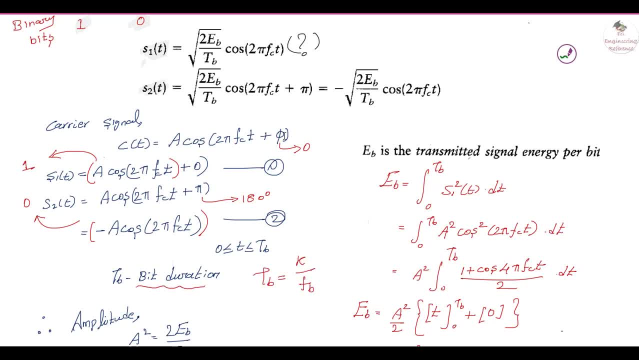 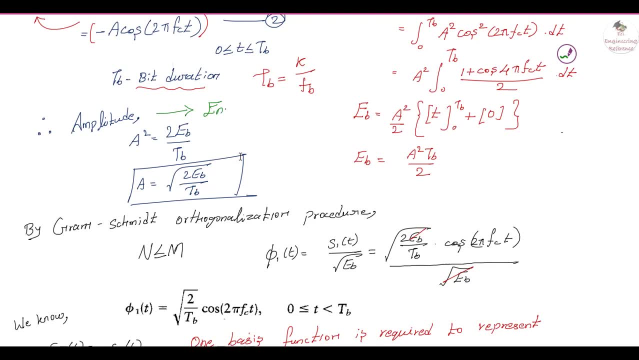 duration. So in the bit duration is generally represented with the integer multiples. So, and in digital modulation we represent that amplitude in terms of energy. So energy here is equal to 0.. And in digital modulation we represent that amplitude in terms of energy. So energy here. 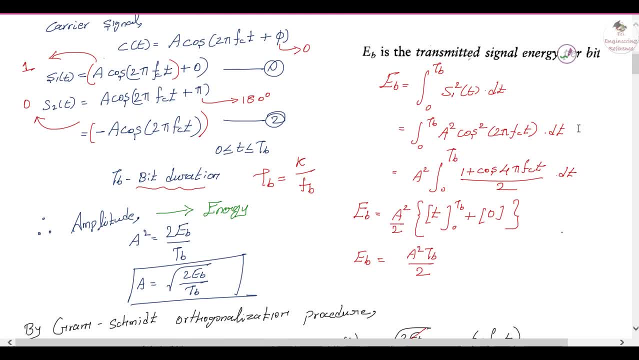 is given, as in the transmitted signal, energy per bit that is given as eb is equal to integral 0 to tb. s1 square. Let us integrate the first signal under the interval of 0 to tb. So energy of the signal is obtained by integrating the square of the signal under the bit duration, So here s1 of. 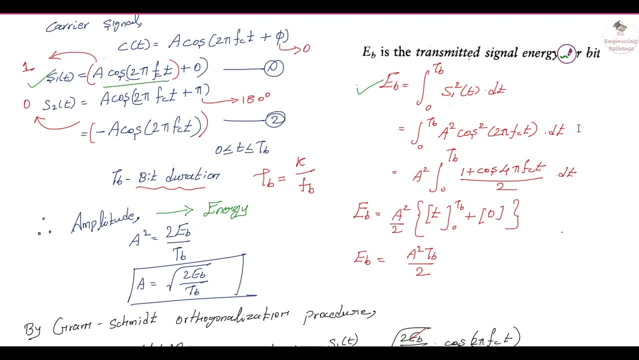 t is a cos 2 pi fct. So substituting here we get a square cosine square 2 pi fct into dt and taking a square outside the constant value we know the cos square theta is equal to 1 plus cos 2 theta. 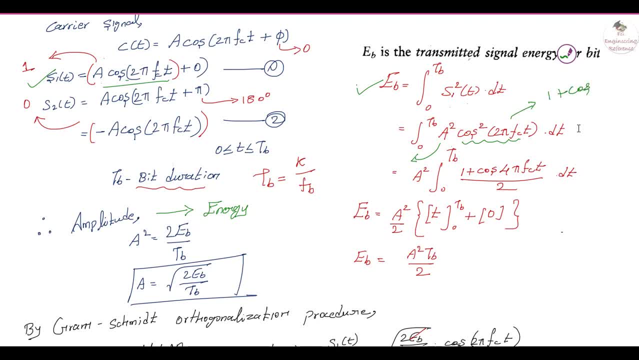 divided by 2.. 1 plus cos 2 theta divided by 2.. So applying this here, we get 1 plus cos 4 pi fct divided by 2 and taking 1 plus cos 2 theta divided by 2 and taking 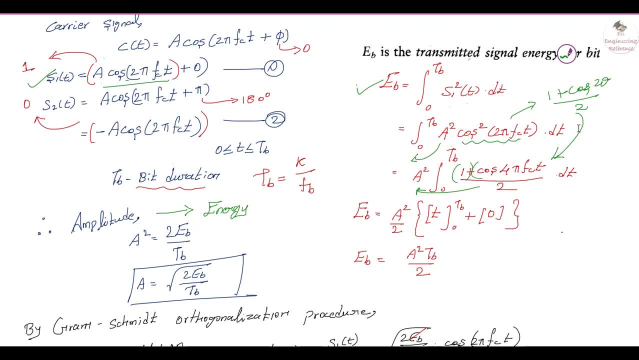 2 outside, integrating 1 and integrating cos 4 pi fct. So integration of cosine 4 pi fct is 0 and integration of dt is resulting as t under the interval 0 to tb. and substituting here we get a square divided by 2 into tb minus 0. So it is a square tb divided by 2.. So that is what written. 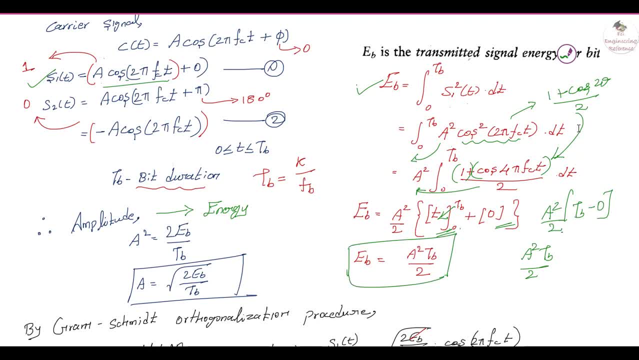 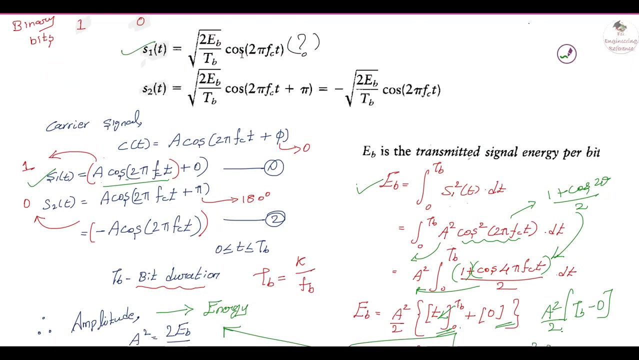 here. So the energy of the bit duration is a square into tb divided by 2.. And in terms of amplitude and rewriting this equation, So a square, rewriting this equation- is a is equal to under root 2 into eb divided by tb. So this is what mentioned here. So the signal s1 of t is under root 2 eb divided. 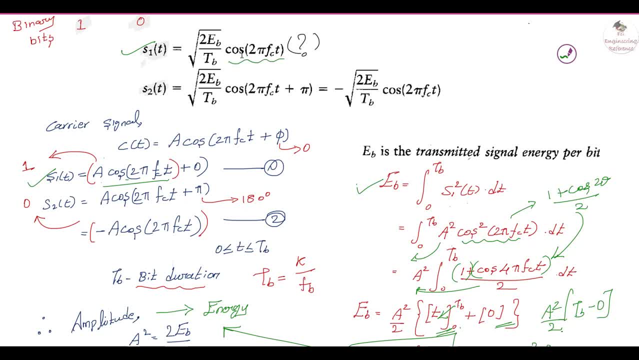 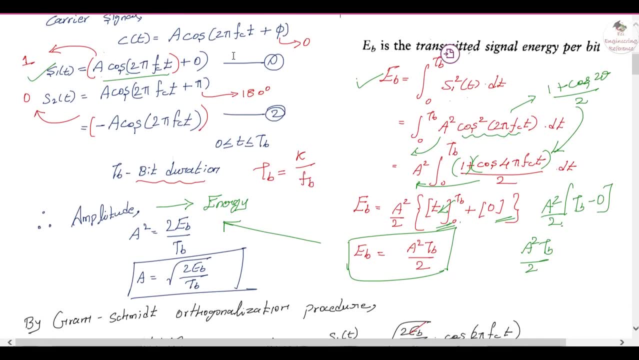 by tb, cos 2, pi, fct, and for the bit duration is a square into tb divided by 2.. So this is what written here. So the signal s1 of t is under root 2 into tb minus under root 2 eb divided by tb, cos 2, pi, fct. 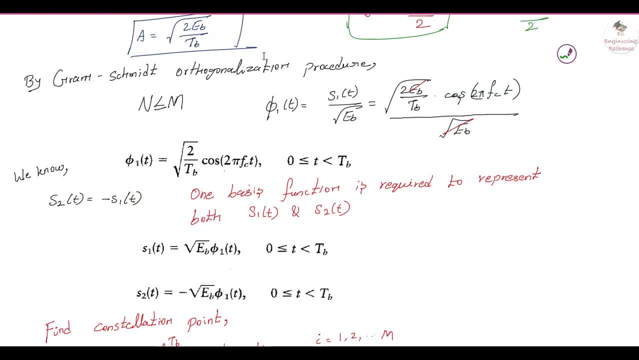 So this is the signal representation and we need to find the basis function in modulation. in every modulation we find the basis function and by using Gramm-Schmidt orthogonalization procedure we can calculate the basis function. Here n is basis function and m is number of signals transmitted, and the condition is: 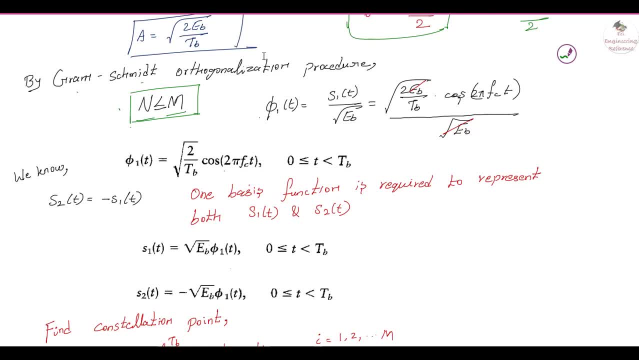 is n less than or equal to m. So the first basis function is calculated as dividing the signal, the first signal, s1 of t, by under root e b. So we get here as s1 of t is written here under root e b. 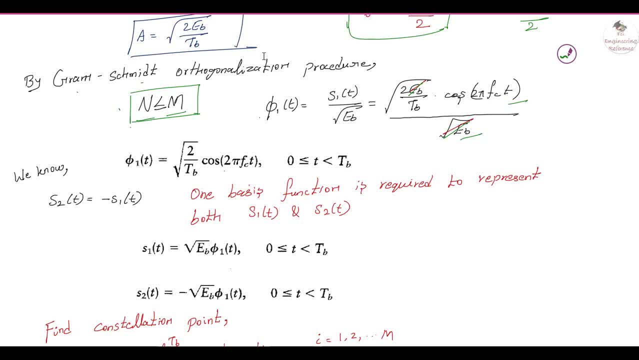 and root e b is getting cancelled. So we are getting the first basis function as under root 2 divided by t b, cosine 2, pi, m, c, t in the bit duration 0 to t b And we know that s2 of t is. 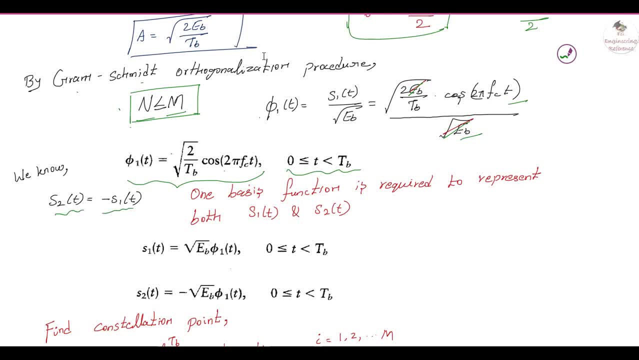 negative of s1 of t And, according to Gram-Schmittthon organization procedure, and pi 2 of t. while calculating based on this method, we will be getting 0.. And we use one basis function to represent s1 of t and s2 of t right. So here n is equal to 1,. 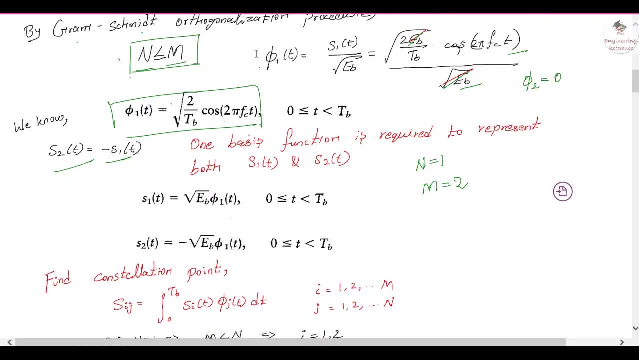 m is equal to 0.. equal to 2.. So the signal s1 of t can be represented. what is s1 of t? it is root eb divided by tb, cosine 2, pi, fct. So taking under root eb outside, right under root eb outside, this can be written. 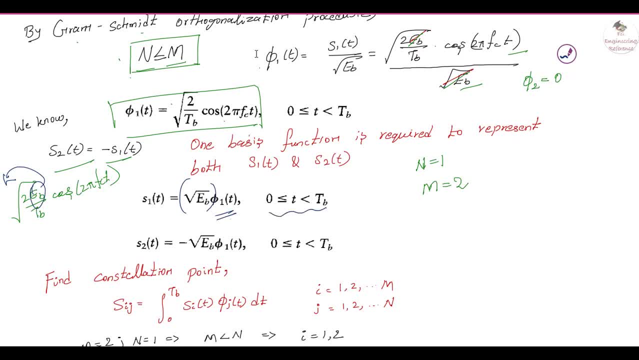 as under root eb into pi 1 of t in the bit duration and signal 2 is represented as minus under root eb, pi 1 of t. So this is the standard signal representation of bpsk signals and this is the one dimensional modulation. Let's see how to find a constellation point. So in general, 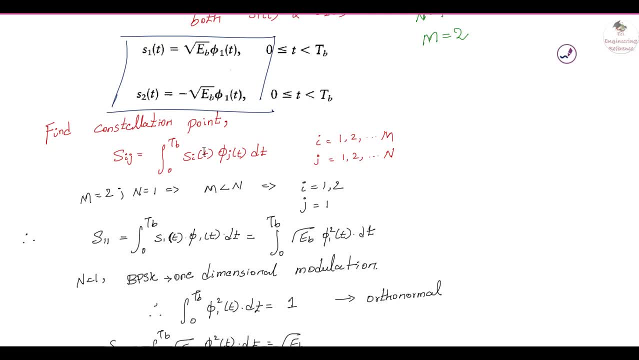 the constellation point is represented as integral of the interval with 0 to tb, that is, si of t into pi, j of t, and i value varies from 1 to m. j value varies from 1 to n. n is the basis function and m is number of signals that is transmitted. So in this context we have two signals, So m is 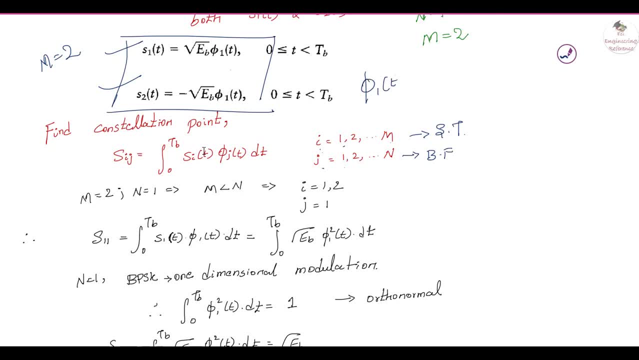 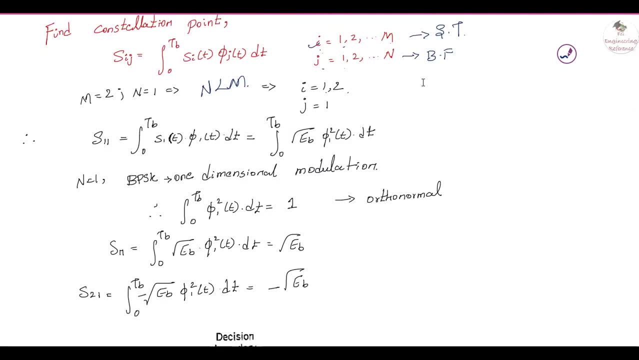 equal to 2 and basis function pi 1 of t So n is equal to 1.. So let us substitute. So i value 1 and 2 and j value here is 1.. So substituting these i and j here in the constellation. 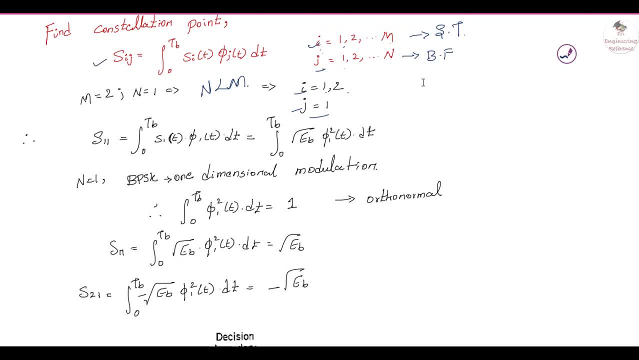 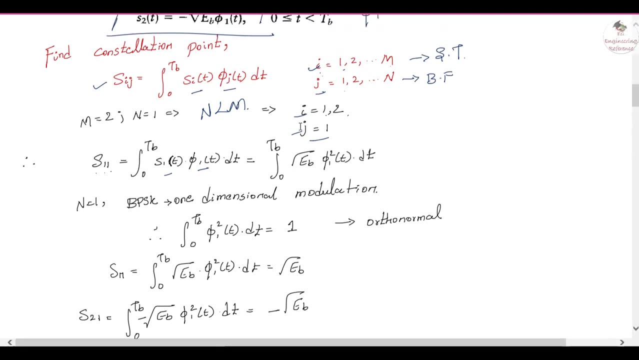 here in the constellation point, equation s 1: 1 and integral of s 1 of t. i value is 1 and j value pi j of t. that is pi 1 of t and substitute s 1 of t. s 1 of t is what, So s 1 of t is under root e b. 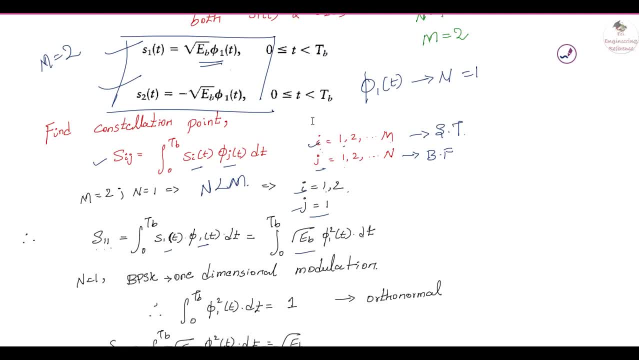 pi 1 of t- right, that is what here written- and into pi 1 of t, which gives us pi 1 square of t. Also, this basis function is of unit energy signal, where that is the integral of the basis function, the energy of the basis function is. 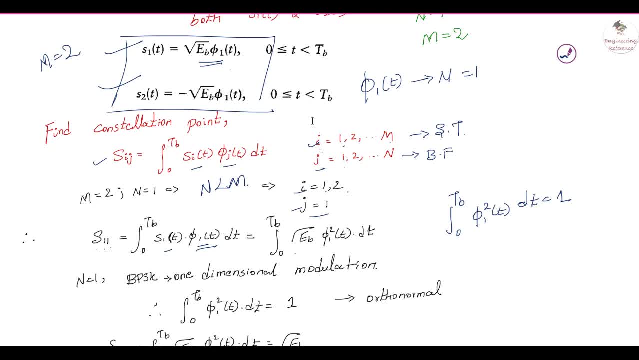 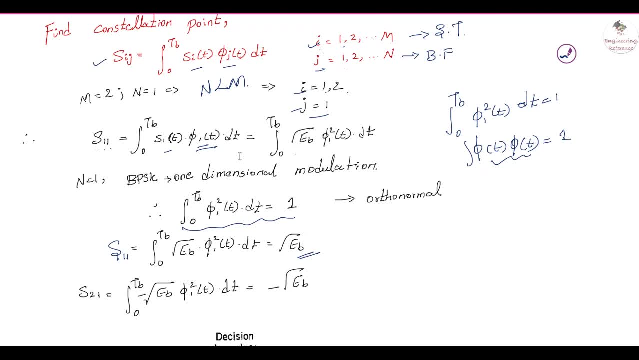 into dt is equal to 1.. So that is what written here s sub 1. 1 is given as under root e, b. with the same way, now substituting i is equal to 2 and j is equal to 1, we get s sub 2. 1 is minus under. 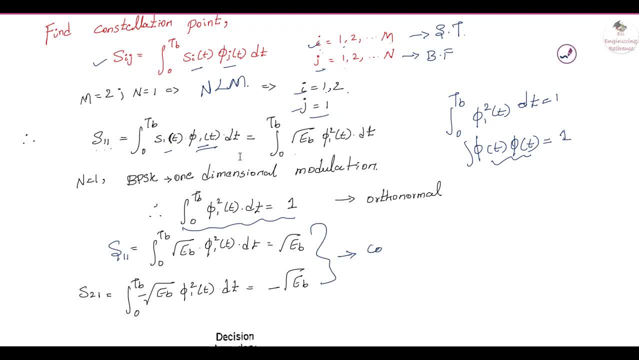 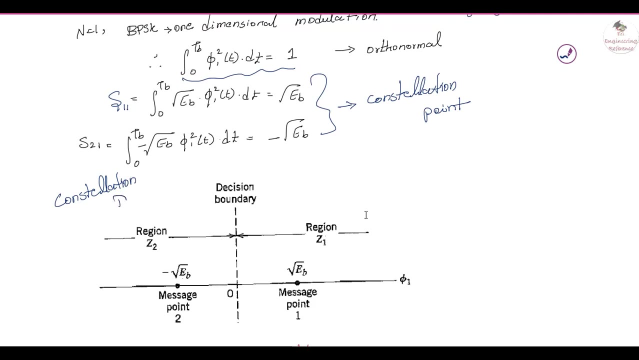 root e, b. So these are the constellation point. These are the constellation point where the received signals are going to be mapped with these energy levels. So here the constellation diagram is shown. We know this is a one dimensional modulation where n is equal to 1.. That is, we are having 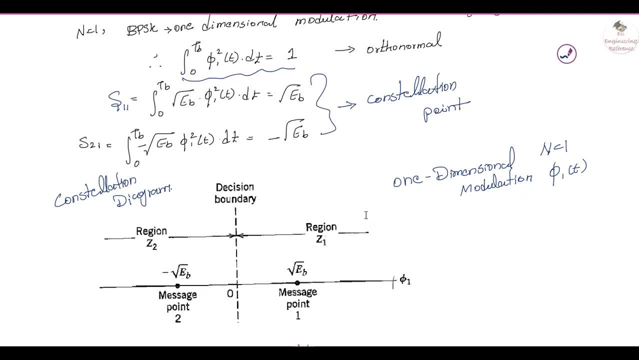 only one basis function. So the basis function is represented here and we have a threshold point. We consider the threshold value, the decision boundary is 0 and from 0 to infinity, whatever the values in these region we can, we take the region 1 z z 1 and region 2 z two, So whatever. 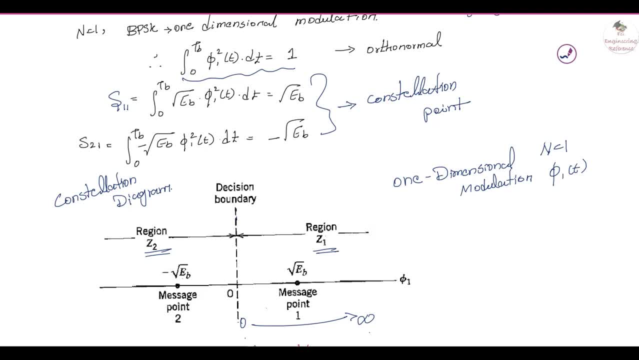 the value. So the values from zero to infinity in this region are going to be mapped to under root e b and the values from 0 to minus infinity in this region are going to mapped to the energy minus under root eb. so under root eb is representing logic one and under root 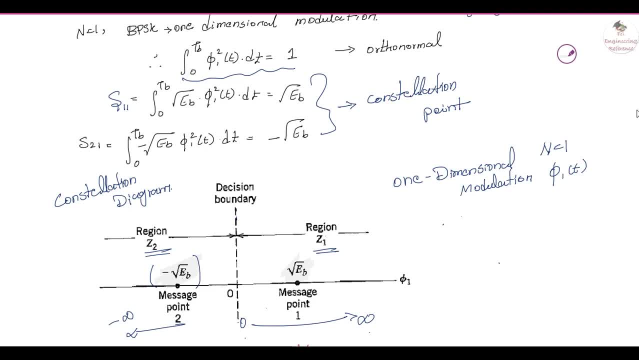 minus eb is the representation of logic zero. so this is how the signals, the message signals- let's say zeros and ones- are mapped. logic one and logic zero are mapped in one dimensional way. so at the receiver side we are having a decision circuit. so based on this, based on this threshold, 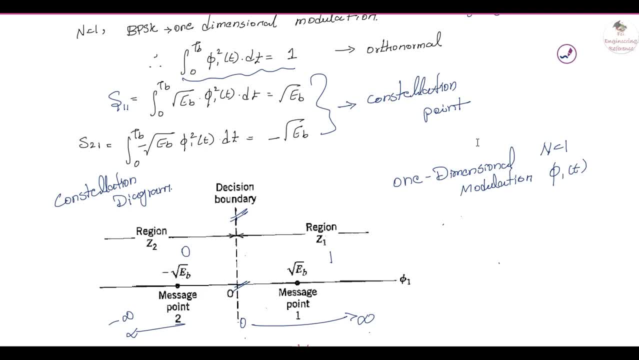 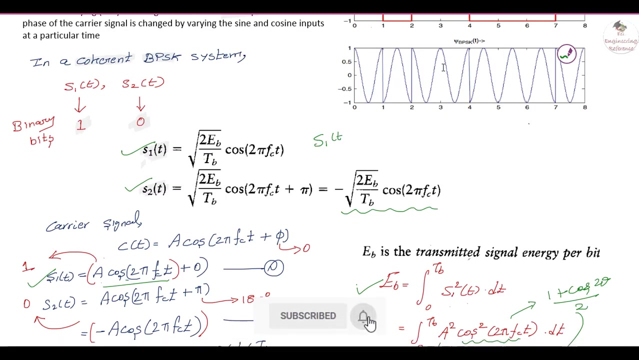 range. if the receiver signal is greater than zero, then the information is extracted as one. so then the information is extracted as one, and if the receiver signal is less than zero, then the information is extracted as zero. and this is how the signal s1 of t is represented as: 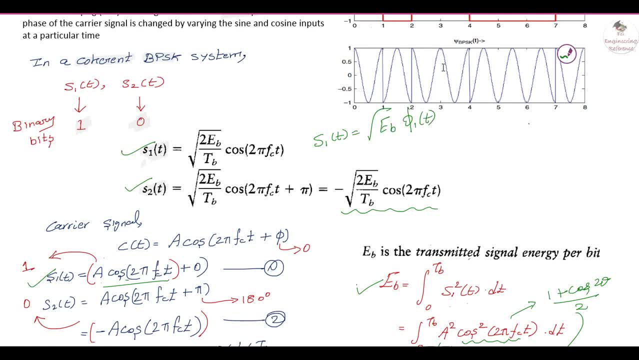 under root eb into the basis function pi 1 of t and the signal to represent this is logic one. and this is to logic. zero. s2 of t in bpsk is given as minus under root eb, pi 1 of t. so this pi 1 of t basis functions are meaning it has a one. 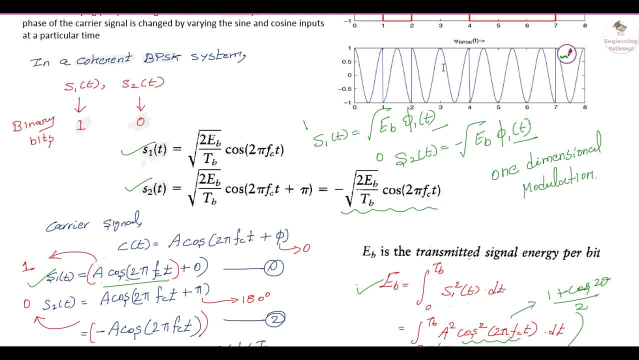 dimensional modulation. so in the next video we will see the transmitter and receiver structure of the bpsk modulation. thank you,